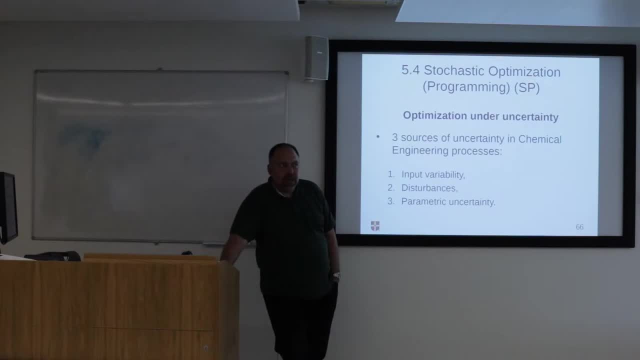 of problems was bi-level optimization problem, ELP, And the motivating example was the manipulation of microorganisms using modeling approaches to over-produce desired products. Today we're continuing with the theme of formulations or general classes of problems that are addressed by optimization formulations, And the first 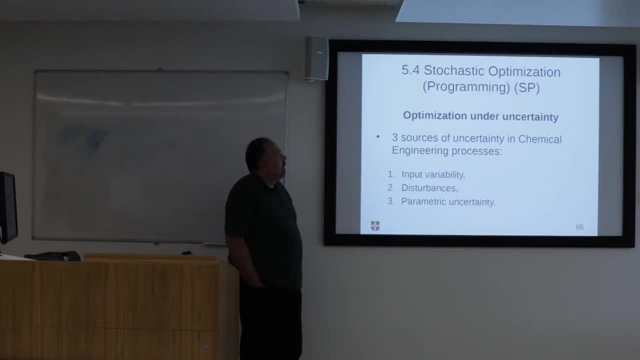 problem we're going to see today is on stochastic optimization problems, Either SP or SOP stochastic optimization problem And it's basically dealing with optimizing systems subject to uncertainty In chemical engineering processes and models. we have, generally speaking, three types of uncertainty or sources of uncertainty. We may have input: 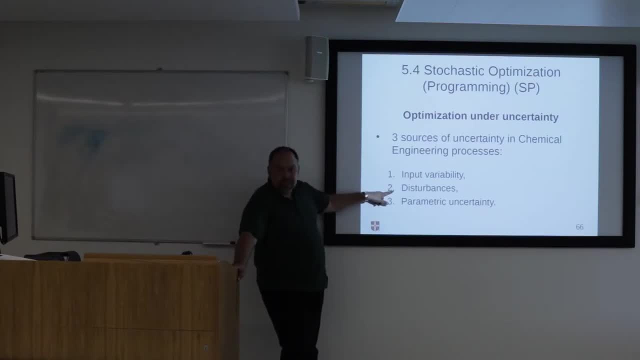 variability, We may have disturbances And we may have parametric uncertainty, which is the bigger class, I think, of problems we have to deal with. For example, when you're designing a plan, you don't know exactly the kinetics, You don't know exactly all the 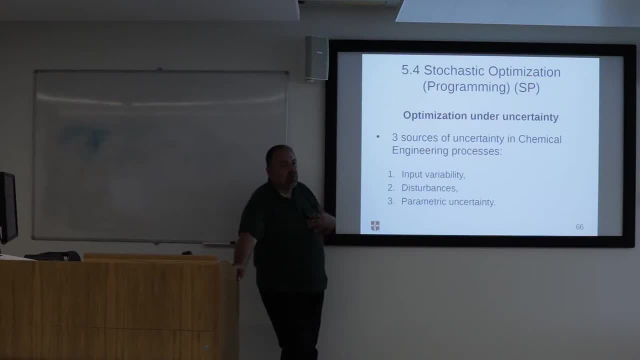 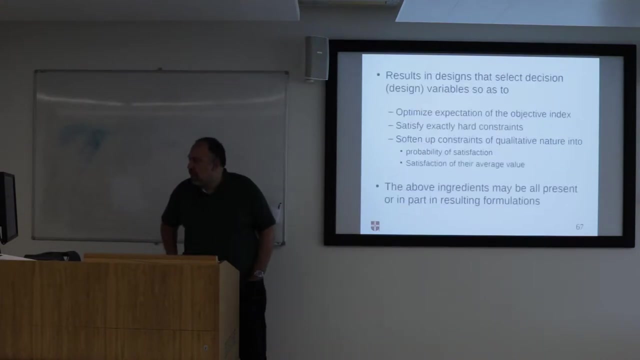 physical properties And therefore you would like to be able to gauge the impact they have on your investment and on the processing ability or operability of what you will act on, And so we're going to look at some of the up designing and implementing. So, if you consider uncertainty within your 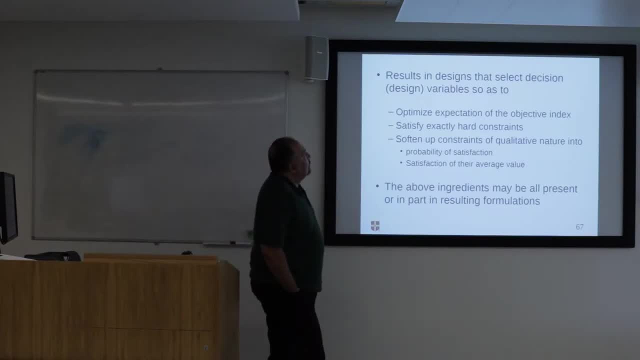 modeling. then it results in designs that select decision or design variables so as to optimize the expectation of the objective function value or the objective index. You don't have a single value because now your parameters are stochastic variables, the random variables, and therefore you expect a. 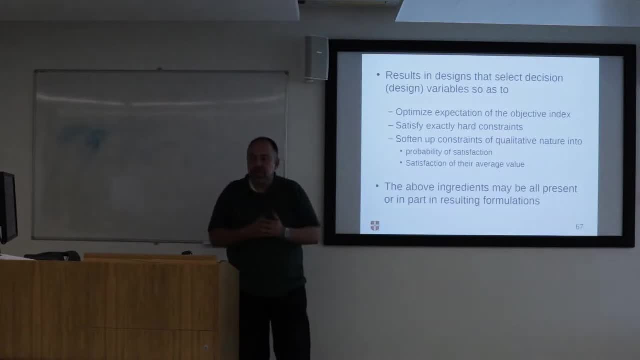 distribution of values of the objective to actually be the result of this, and you may have to soften up constraints of qualitative nature into either probability of satisfaction of those constraints or satisfaction of their average value. The above ingredients may be all present or in part in resulting. 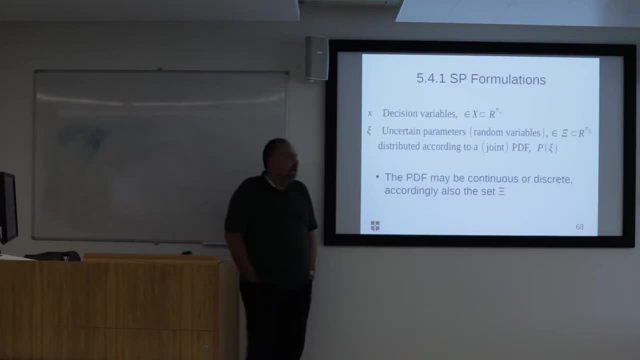 formulations. So let's look at some stochastic programming formulations. You have, as usual, your decision variables x, n in number, n, x in number, and you may have your uncertain parameters, which are random variables. xi are distributed according to a joint probability density function. The PDF may be continuous or 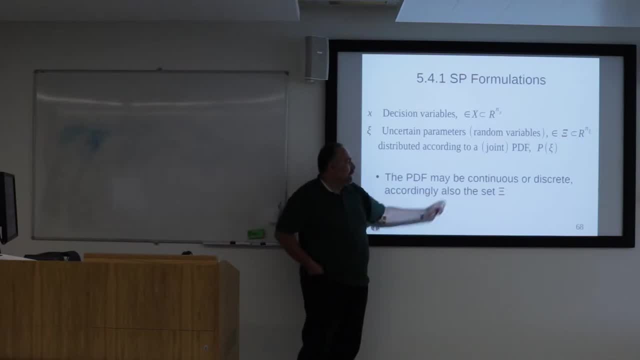 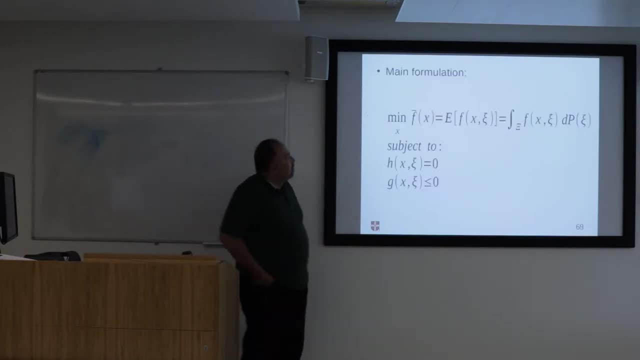 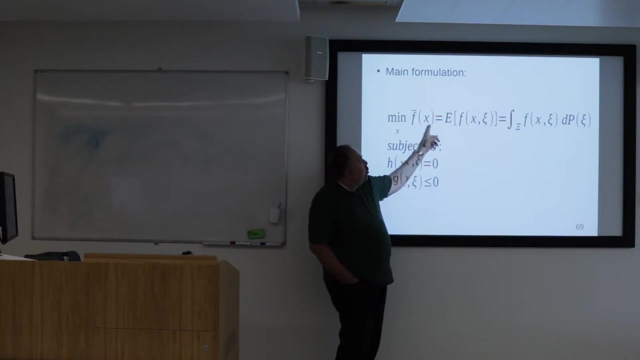 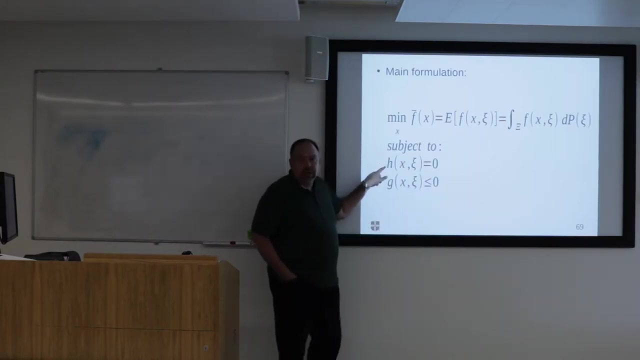 discrete are also the set, the big set Xi, to which the random variables belong to. So the main formulation is as follows: We want to minimize a performance index, f hat, which is the expected value of your actual performance index with respect to X, and it's subject to the usual equality and inequality constraints we have. 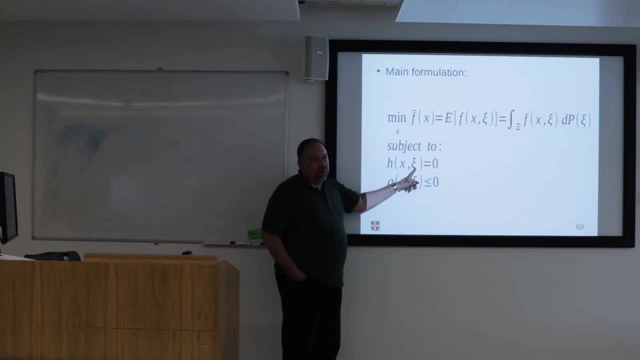 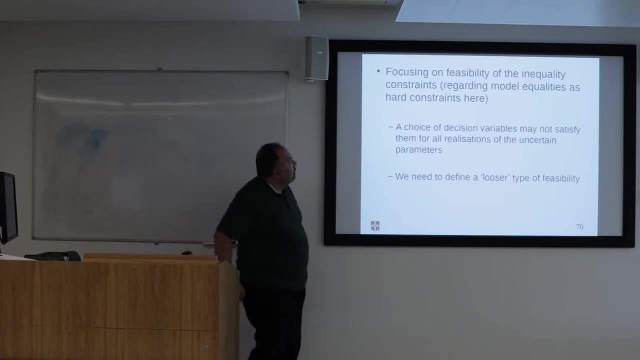 before. The only difference here is that they have extra arguments, which are the random variables, the parameters of the model. So focusing on feasibility of the inequality constraints and regarding the model equalities as hard constraints. here, a choice of decision variables may not satisfy them for all realization. 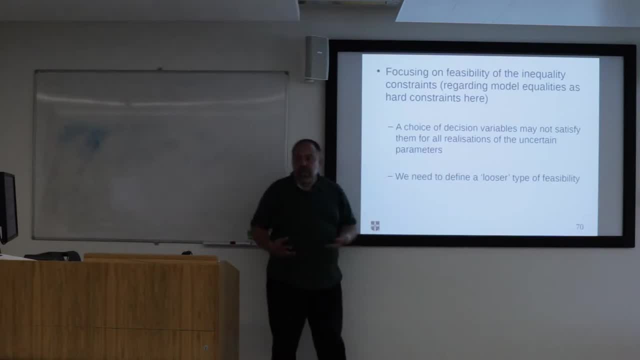 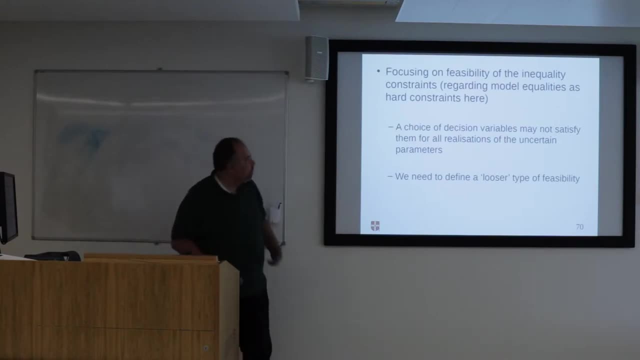 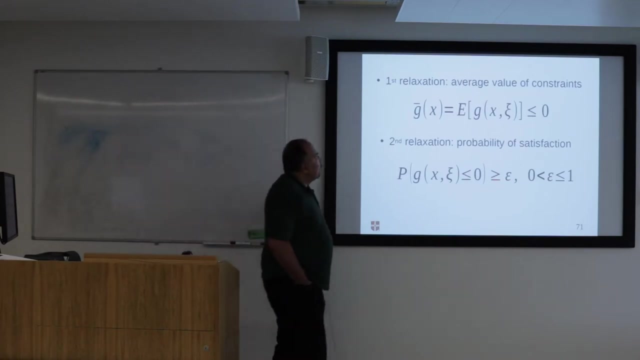 of the uncertain parameters. So basically, choose an X. some of your inequalities may not be satisfied. So what do you do? We need to define a looser type of feasibility in order to be able to derive some solutions that we can apply in practice. So the first type of relaxation is that we do to inequalities. 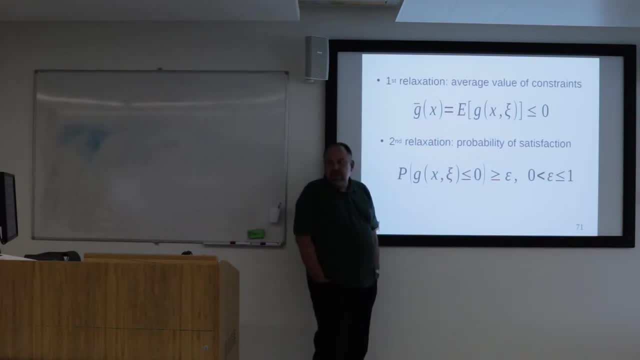 what we did to the equalities of the random variables. So the first type of relaxation is that we do to inequalities what we did to the objective function. We take its expected value, that's the mean value of the constraint with respect to the parameters Xi, and we say that this mean 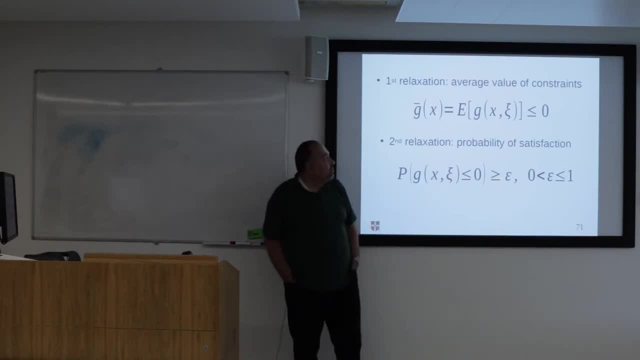 value should be less or equal to zero, Whereas in reality we wanted all G to be less or equal to zero. So that means that some of these constraints- possible combinations of X and Xi- will result in infeasible constraints. So that means that some of these constraints- possible combinations of X and Xi- will result in infeasible constraints. 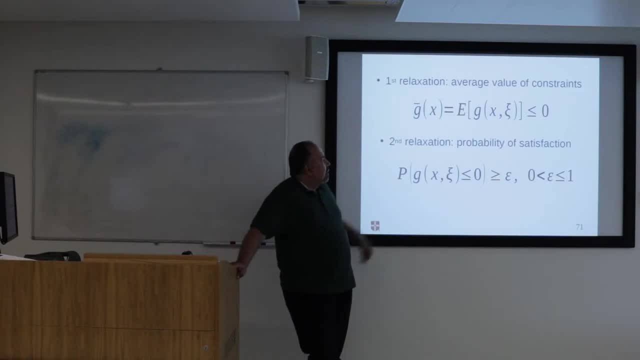 constraints with this. Then the second type of relaxation is the probability of satisfaction of the constraint, or this has another name, which is called chance constraints. Basically, what you do is you say that the probability of the inequality constraint to be less than zero- I want it to be greater than some. 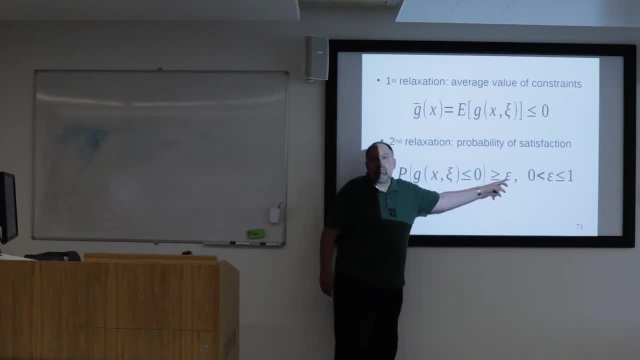 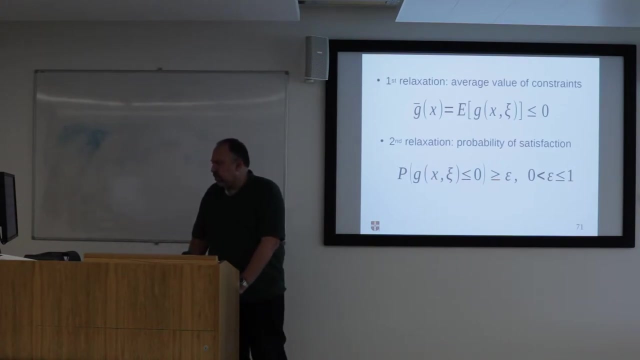 minimum probability epsilon, So this could be 0.95 or even tighter, 0.99% of the time. Again, this means, though they may have some realizations for the random variables Xi that are not feasible, But at least you know the probability of that happening. For example, safety constraints could fall. 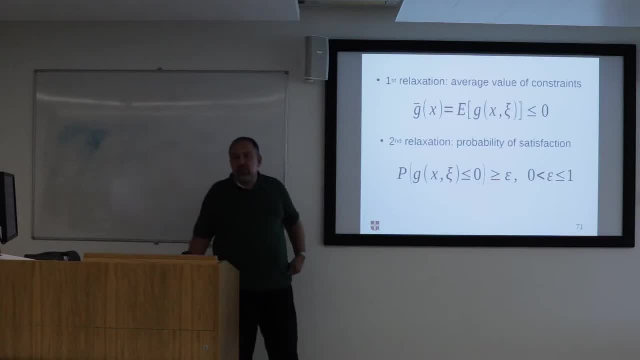 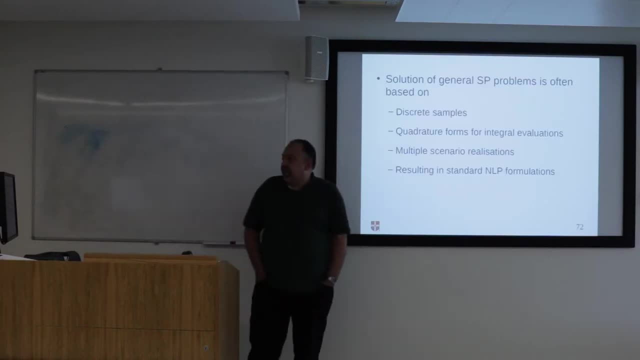 into this type of formulation where you put a tight probability of them not happening, not being feasible. So how do we solve these problems? Well, their solution of the solution of general stochastic programming problems is often either based on discrete samples, So we create scenarios where we sample from the PDF several scenarios of the values. 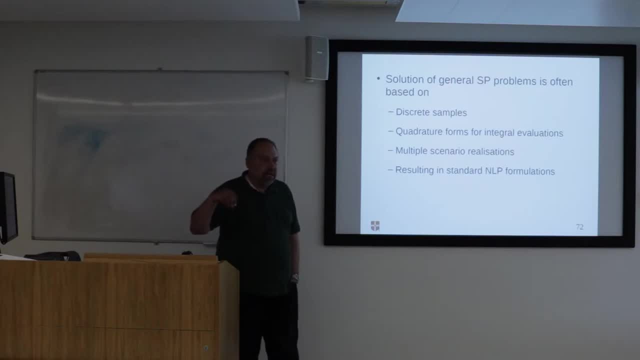 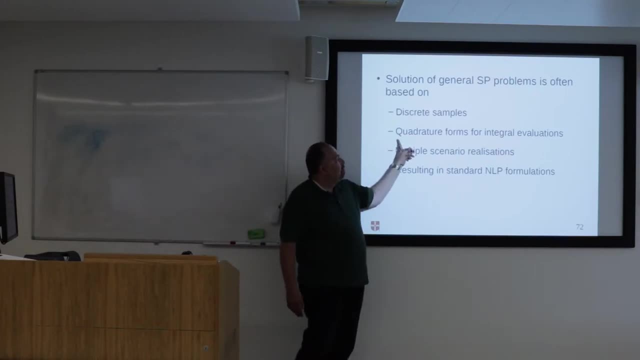 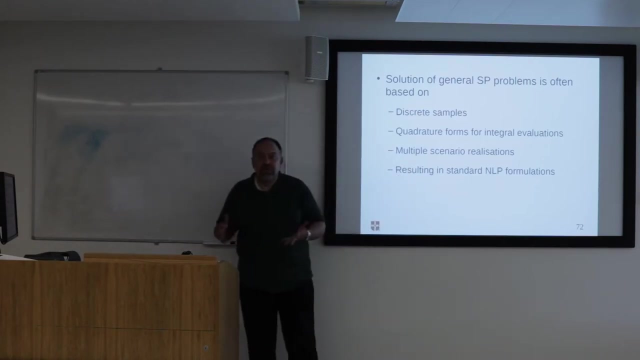 of the randomly distributed variables, parameters Xi, and we create instances which we solve simultaneously, Use quadrature forms for integral evaluations. I talked about the multiple scenarios and basically what you're trying to do at the end of the day is to transform the problem into something that you can solve with conventional 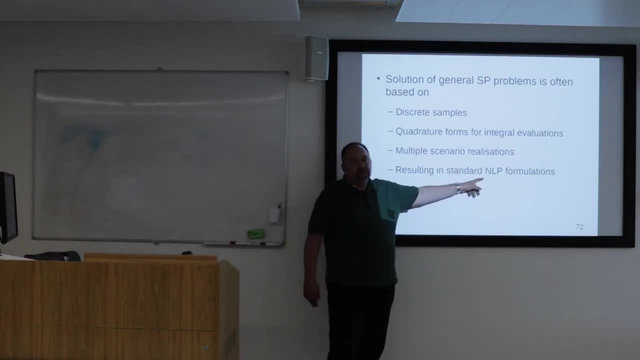 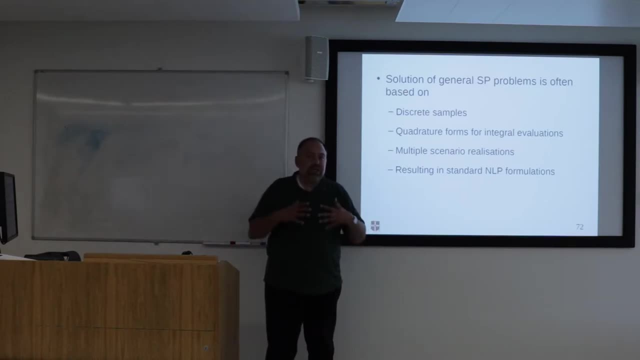 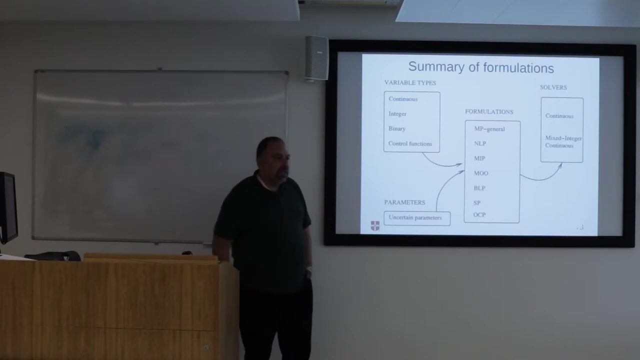 solvers, such as nonlinear programming solvers, And therefore you reformulate with whatever technique you use your problem into a standard nonlinear programming problem and you try to solve that in that way. I've got a question. Can you go two slides before? Once you apply the second relaxation? 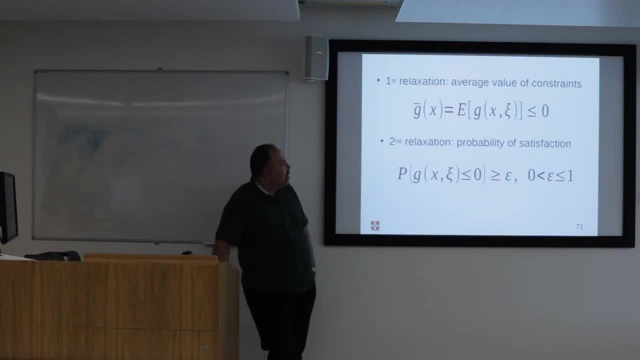 This one. yes, I think the first relaxation is inclined, Say epsilon to be 0.99.. It depends on your epsilon, Okay, I suppose. So this means that if you have a large enough epsilon, say more than 0.99. 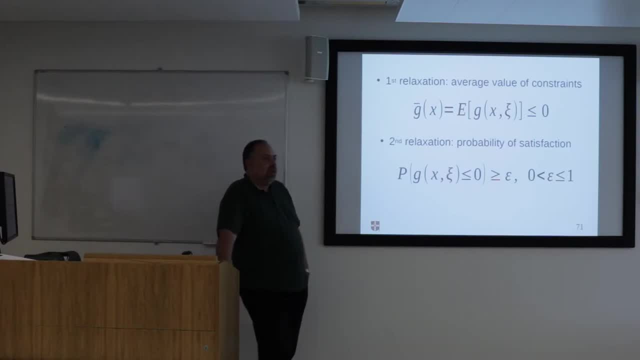 Yeah, First relaxation is included in the second one, Or do we explicitly need first and second one to have both? You wouldn't use both, I think. Not entirely sure what happens in this case. I haven't thought about it, Okay. But, 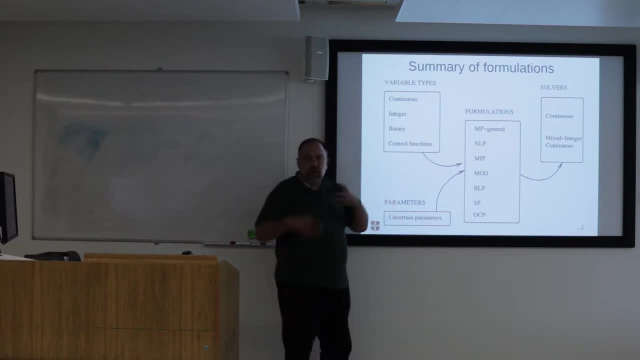 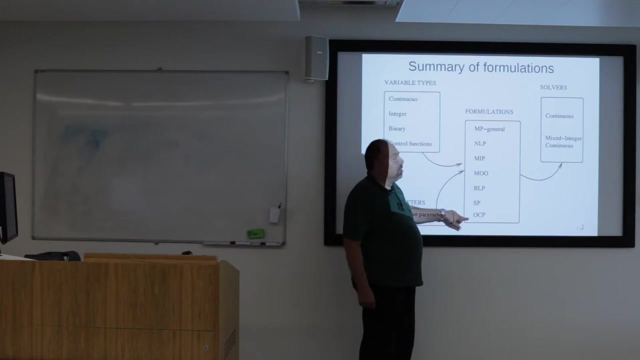 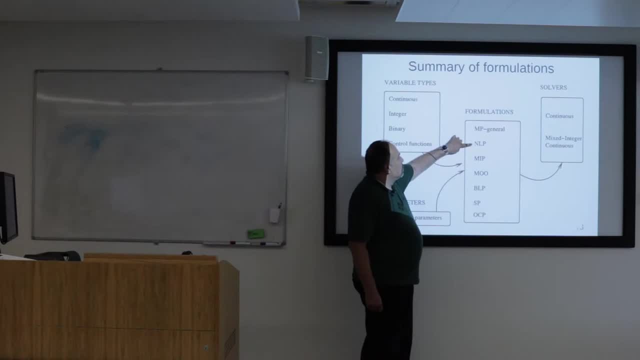 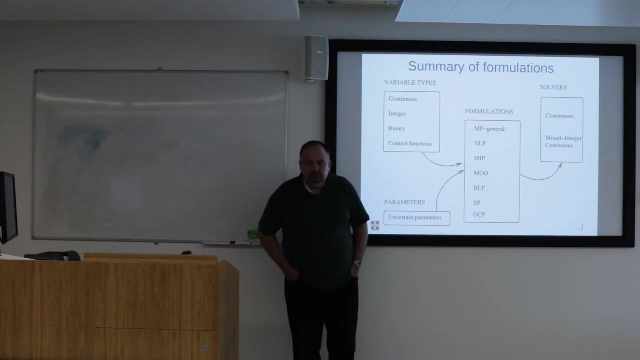 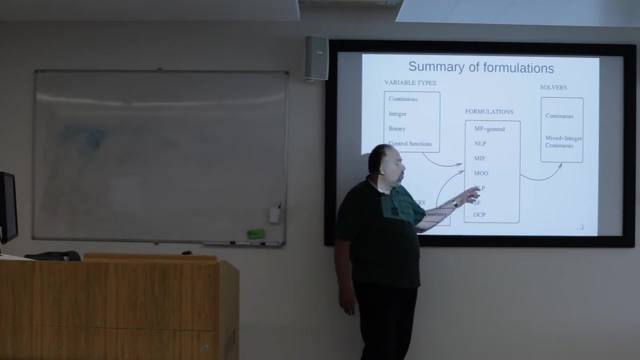 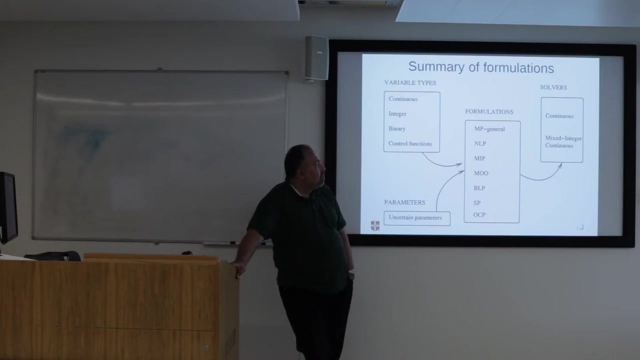 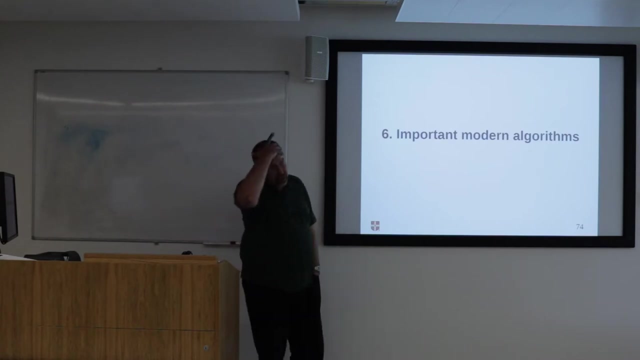 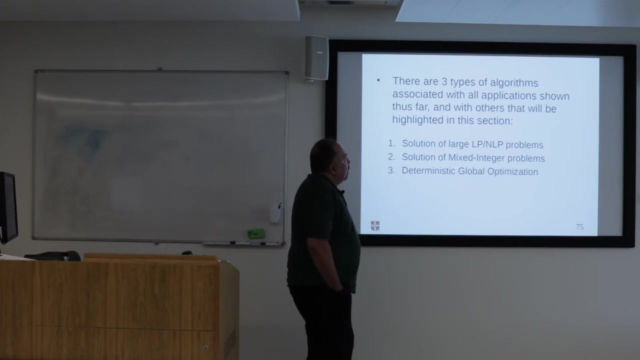 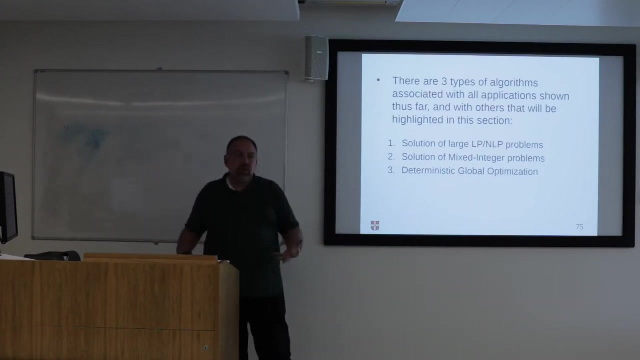 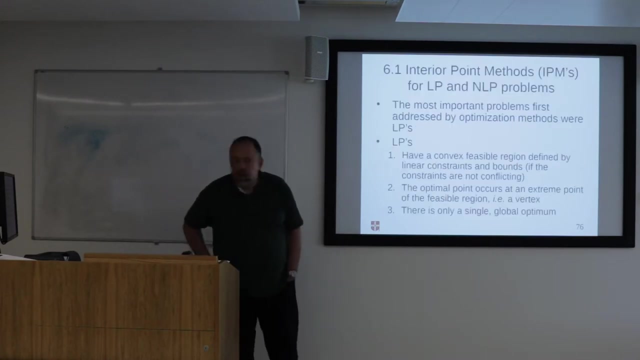 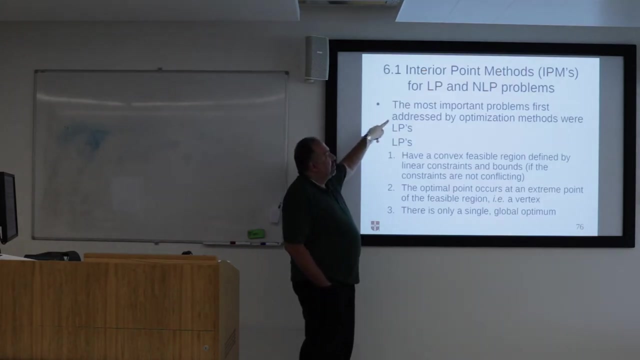 Therefore, true load restoration is what are called interior point methods for linear programming and non-linear programming. These are the most important problems. first addressed by optimization methods were linear programming problems. Lp's have the following properties: they have a convex feasible region defined by linear. There are constraints and bound once. if the constraints are not conflicting, uploading. 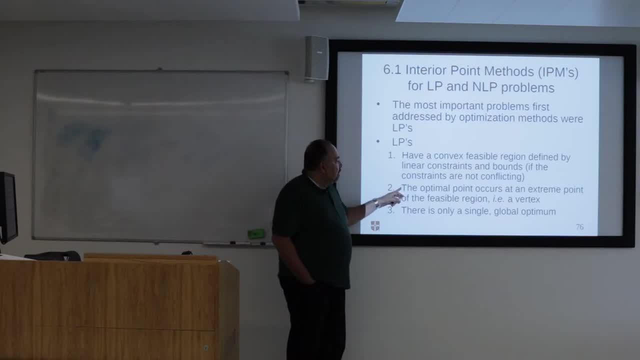 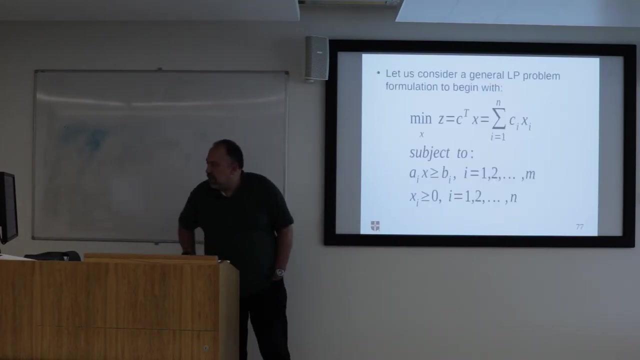 therefore you have a non-empty feasible region. The optimal point occurs at an extreme point of the feasible region, ie a vertex, because of the linearity of the constraints and there is only a single global optimum to such a problem, So a 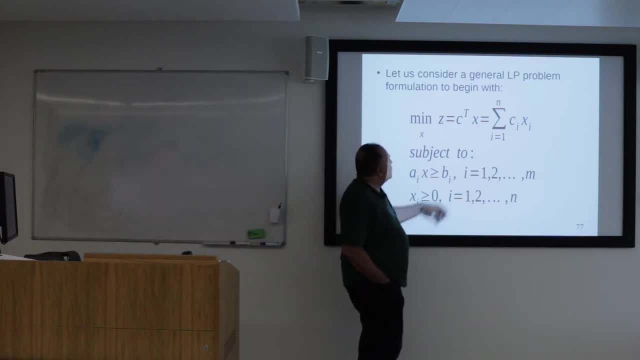 general LP problem is formulated like this: C is a vector of constant coefficients which go into your objective function. x, i are your continuous variables that you want to choose optimally and they're subject to linear inequality, constraints and bounds, non-negativity bounds. This is a simple. 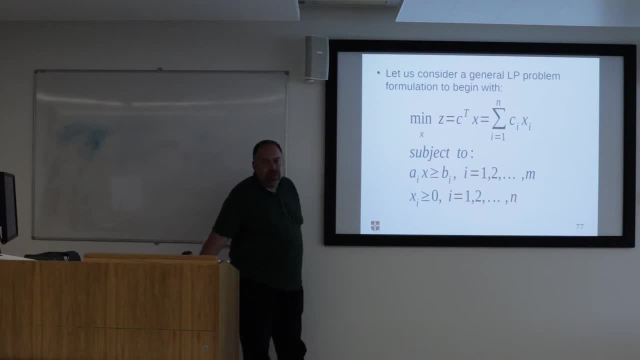 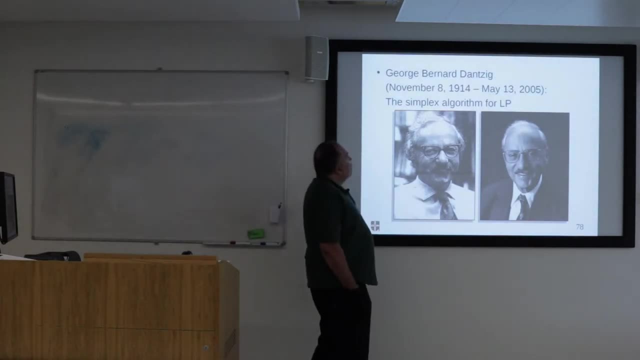 formulation but general enough to demonstrate what I'm trying to show. So the problem is that you have a non-empty feasible region, ie a vector of constant coefficients because of the linearity of the constraints, and there is no solution to it. You have to come up with a solution that is linear and 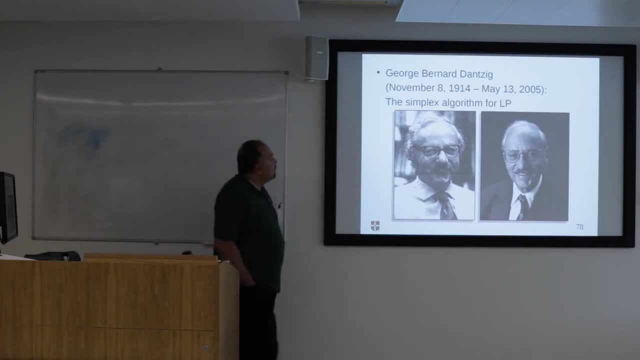 based on that, you have your un-empty feasible region, ie a vector of constant coefficients, and it's the non-empty feasible region. So the problem is this: is that you're going to have an un-empty feasible region with the independent power of the linear algebra. that is the non-empty feasible. 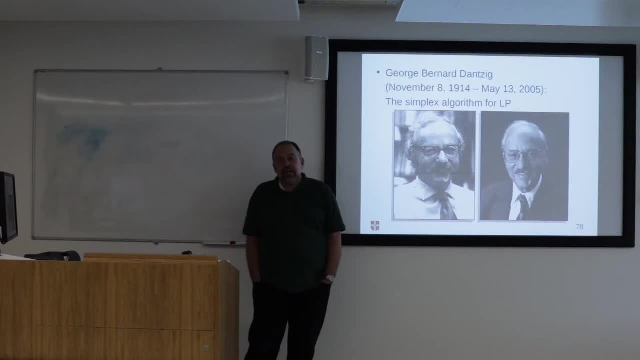 region, And so what I'm trying to show, what I'm trying to show- is that you can do the same thing over and over. You can do this by using the assumption of linear development as a solution, And so this allows the argument of linear. 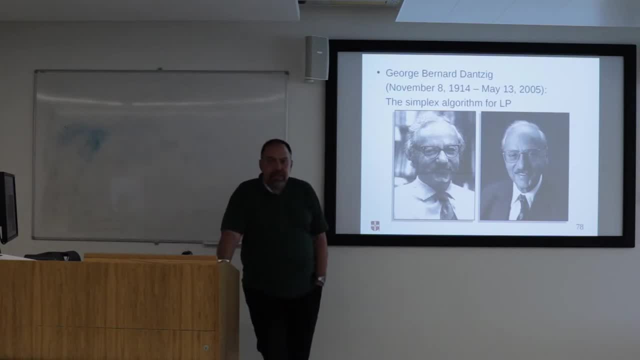 invented? well, he worked on linear programming, definitely, but he invented a solution technique which was held secret then by the Soviet Union and then was later used to minimize losses in their army and maximize losses to the enemy. But nonetheless, the father of linear programming is. 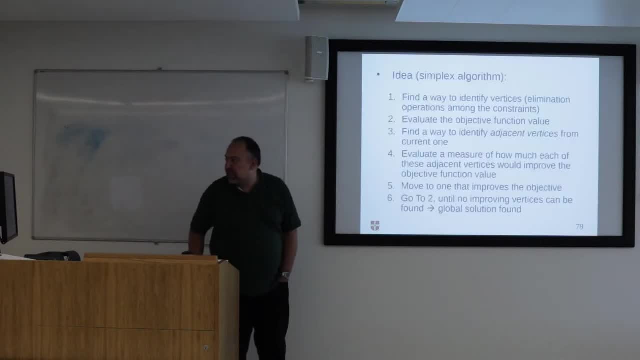 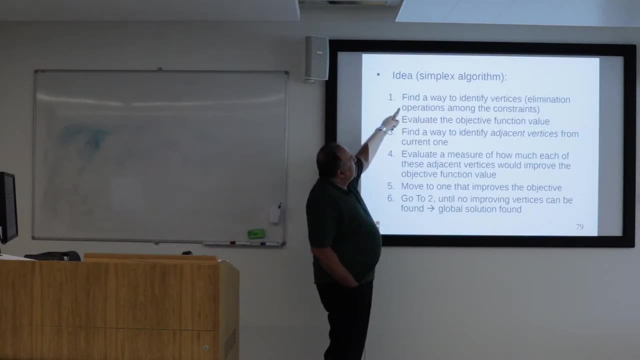 considered to be George Danzig with his simplex algorithm. The simplex algorithm is very, very simple to understand. You want to find a way to identify vertices by elimination operations among the constraints. Evaluate the objective function value at a vertex. Find a way to identify. 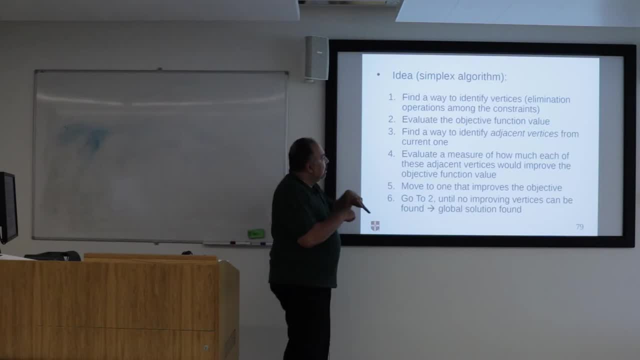 adjacent vertices from where you are. Evaluate a measure of how much each of these adjacent vertices would improve the objective function and move to the one that improves the objective- Anyone that improves it. Go to step number two, which is evaluate the objective until no improving vertices. 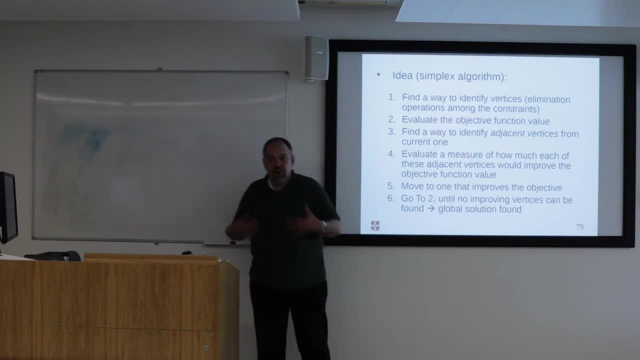 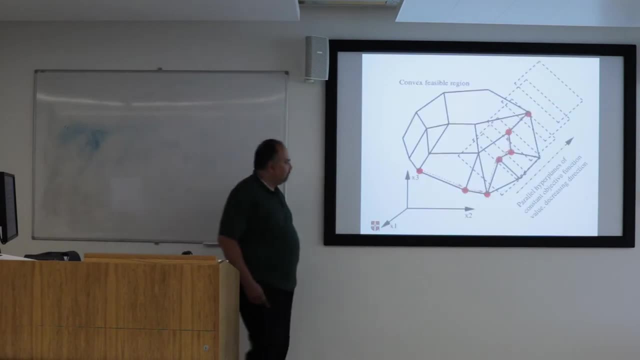 can be found, at which point you have a proof of the optimal solution. It's the global solution. So this is how it works. You start from here. This is the feasible region In general. it's a polytope in higher dimensions which is a multidimensional. 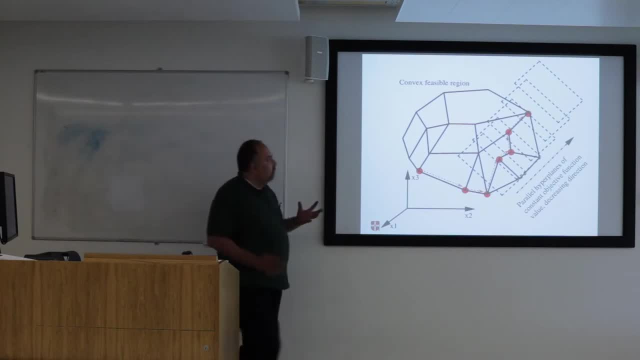 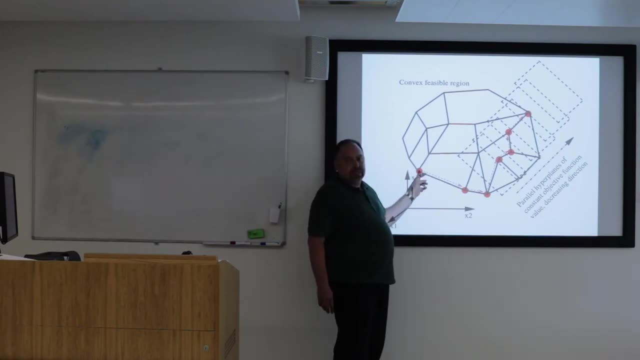 polyhedron. So the solutions we know are to be found on some vertex. So you start at a vertex, provided you identify one, You move to the one that improves the objective, Anyone around it, And you follow the path until you are at a point where to improve. 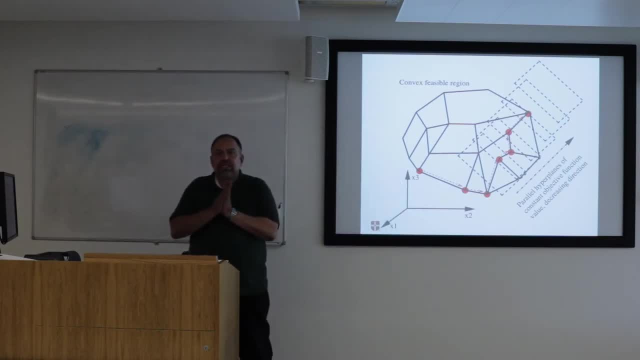 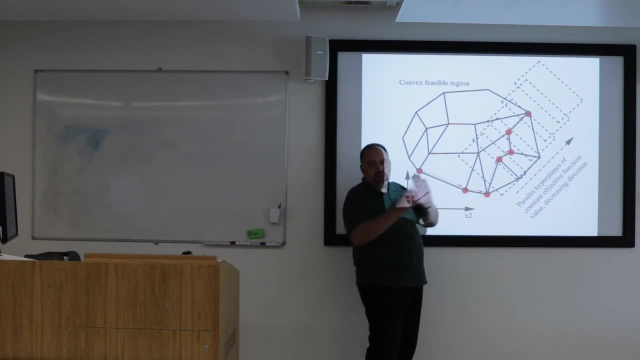 the objective, you would have to leave the feasible space. And you follow the path until you are at a point where, to improve the objective, you would have to leave the feasible space. That's the last vertex which the hyperplanes of the objective function are in contact with. So 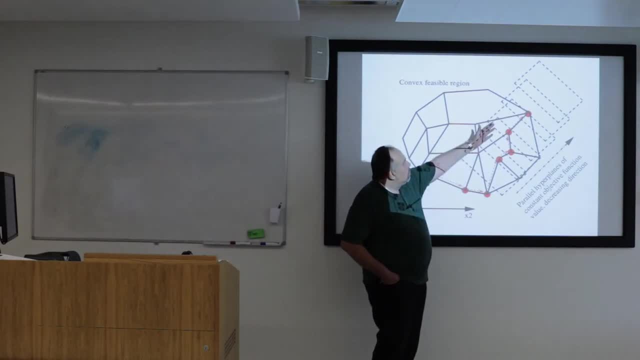 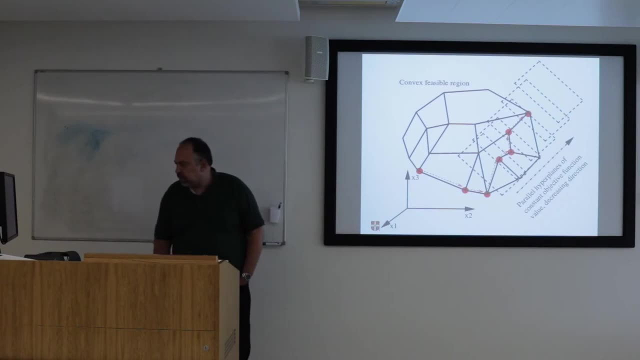 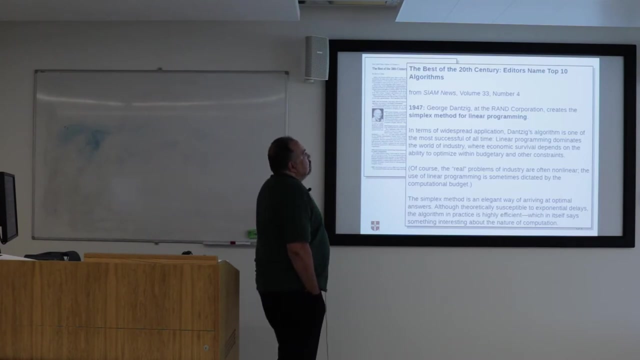 this is the way we minimize the function And therefore, up there is the optimal solution And you stop because you can't find any vertex that improves it. So if we go to see what we published about various algorithms of the 20th century, 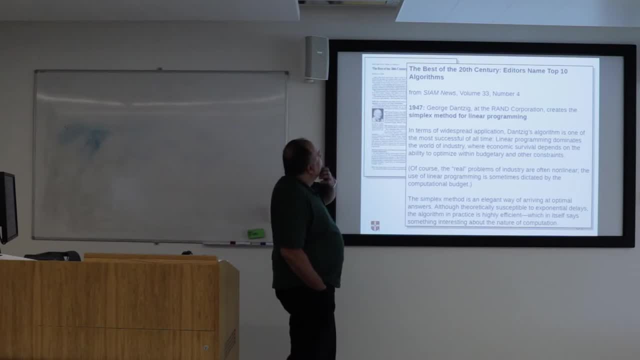 This is SIAM News, Society of Industrial and Applied Mathematics publication. Among the top 10 algorithms, best algorithms of the 20th century, is George Dantzig's simplex method for linear programming. It is interesting to read what it says. It says here that it's one of the most successful of all time because linear programming dominates the world of industry, where economic survival depends on the ability to optimize within budgetary and other constraints. 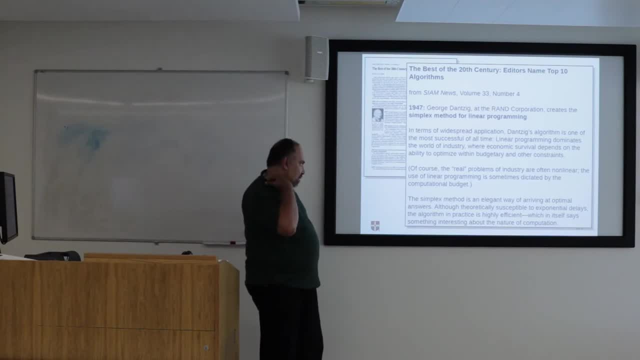 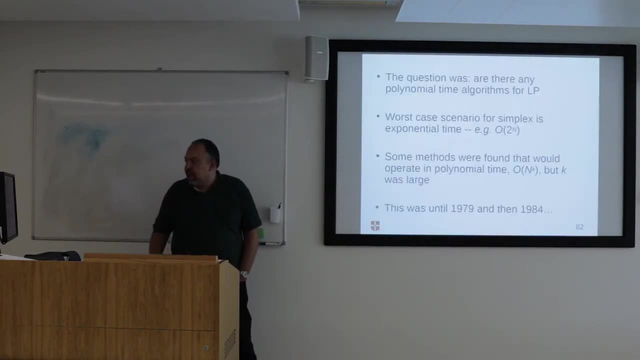 So that's the motivation behind it and why it's very important. Now there was a big question in linear programming. Now there was a big question in linear programming. Now there was a big question in linear programming. Are there any polynomial time algorithms to solve the problem? 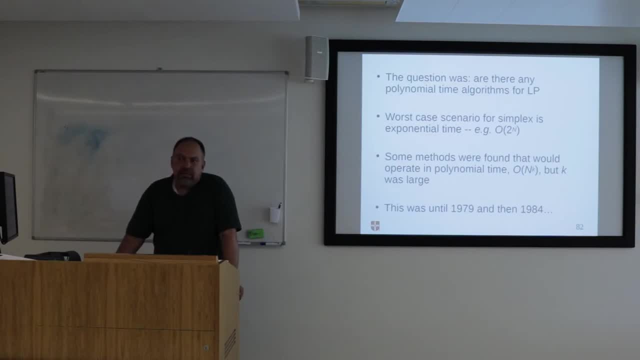 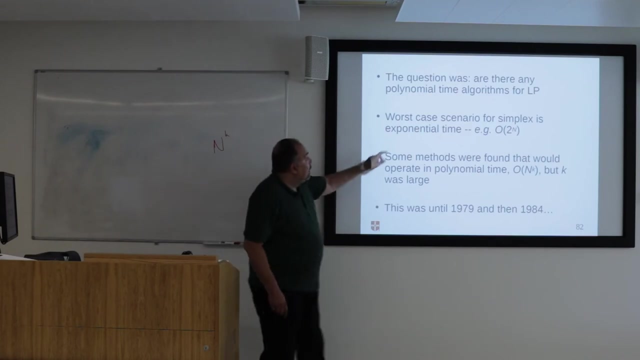 Polynomial time means that, let's say, in terms of the number of variables, if n is the number of variables, is there a low enough exponent, k, which typifies how many iterations the algorithm will need to converge? The worst case scenario for the simplex algorithm with constructed examples is known to take exponential time, not really O2, to the n. 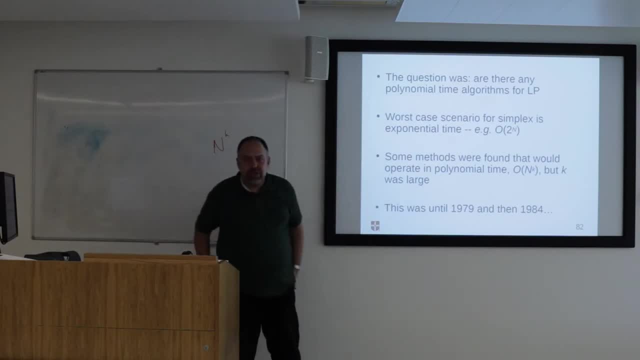 This is an example of what I mean by exponential. It's combinatorial nature in the number of variables and constraints, And there is no known bound for the simplex algorithm. It can perform very badly, although in practice it doesn't do so, for fairly large-sized problems. 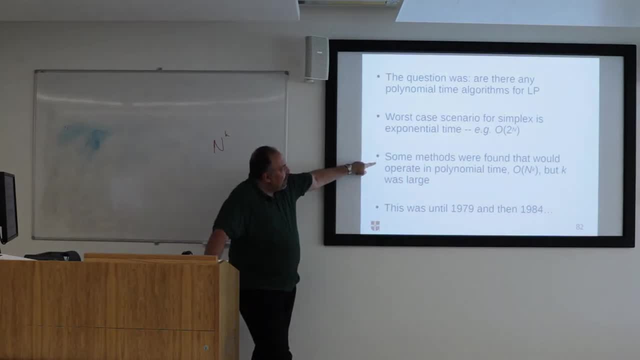 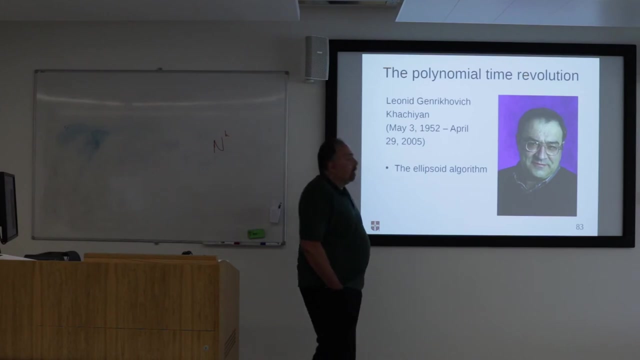 Some methods were found that would operate in polynomial time, but k was very large, And that was until 1979. And then, in 1984, the following happened: It was the polynomial time revolution. It's Due to another Russian mathematician, Leonid Kakian, who died very early in his life in 2005,, who invented the ellipsoid algorithm. 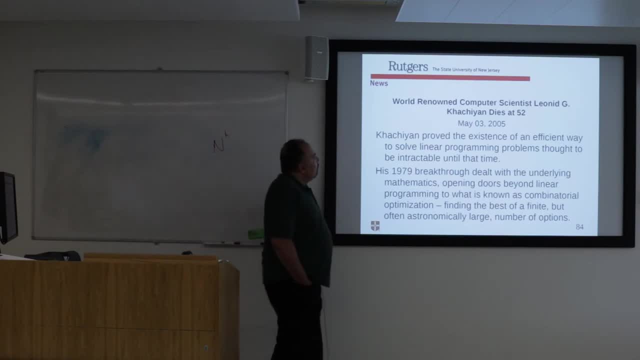 And again, this is from Rutgers and it was the obituary, the announcement of the death of Kakian, who proved the existence of an efficient way to solve linear programming problems. And again, this is from Rutgers and it was the obituary, the announcement of the death of Kakian, who proved the existence of an efficient way to solve linear programming problems. 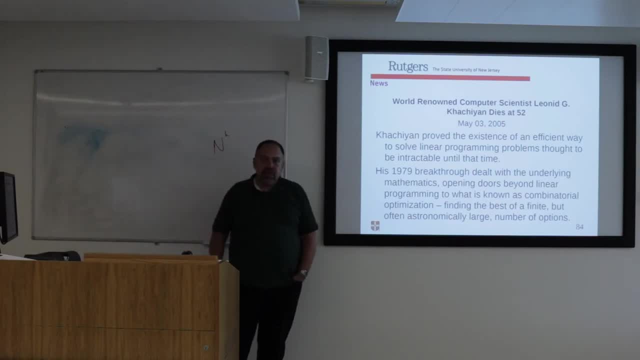 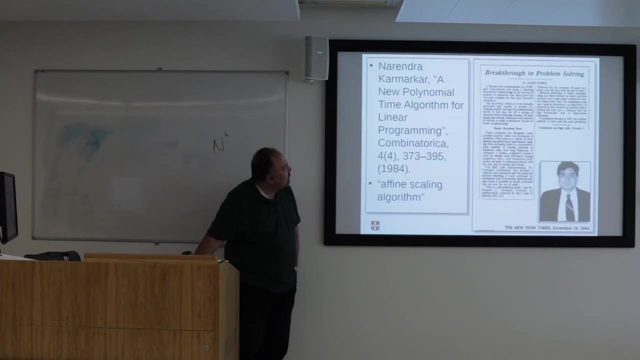 Thought to be intractable up to that point. Again, I repeat, the simplex algorithm in practice performs really well, But the worst case scenario is exponential time. So, moving on from this, another thing happened In 1984, okay, the proof of the ellipsoids by Kakian just proved that there should be. 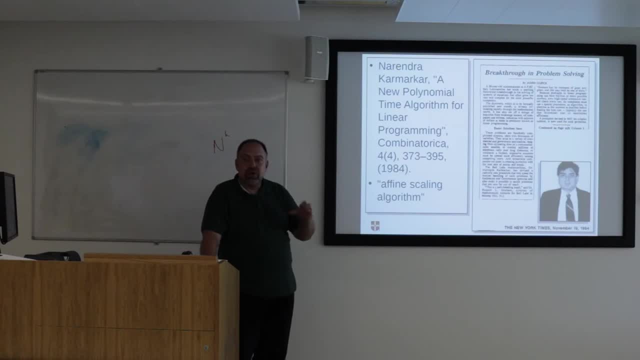 There was at least one way to solve in polynomial time linear programming problems, But there was no efficient algorithm up to that time. This happened in 1984 by Karmarkar's method, which was polynomial time for linear programming, And it was called an affine scaling algorithm. 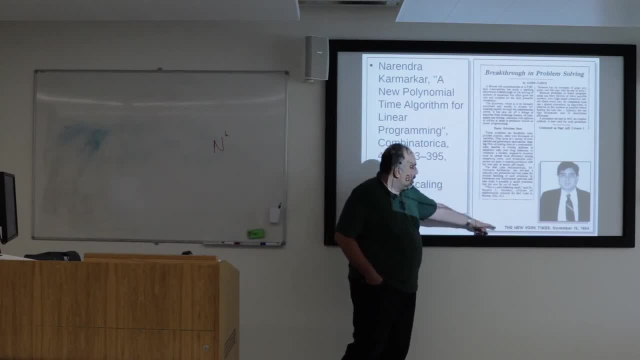 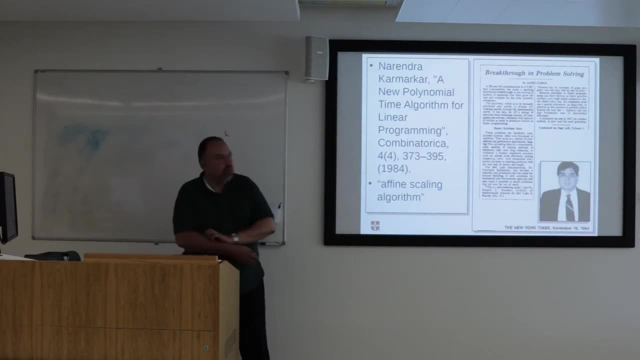 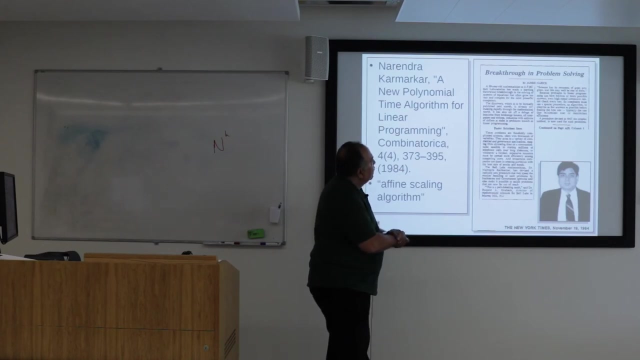 And it even made the news in the New York Times. He- at the time he was 28 years old, it says here- was a mathematician at the AT&T and Bell Laboratories and made a startling theoretical breakthrough in coming up with such an algorithm. Now, 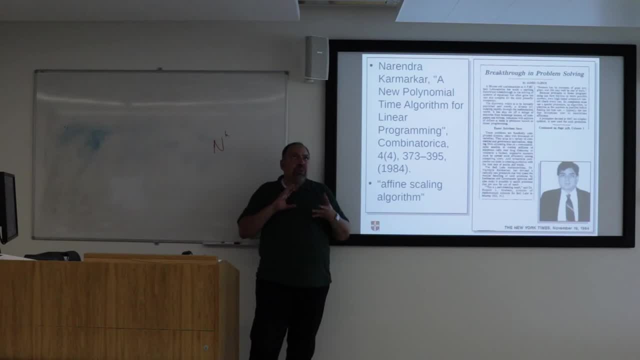 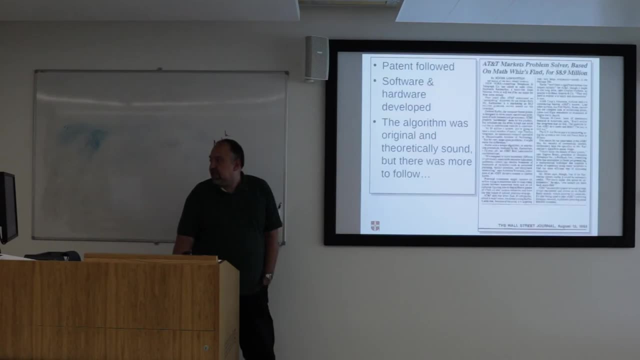 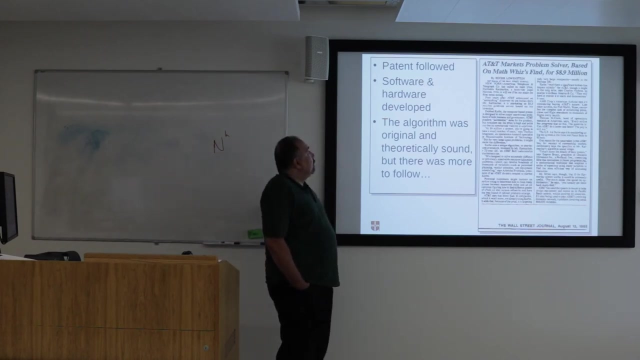 this. a fine-scaling algorithm, is more geometrically inspired, I would say. And then, following this, AT&T created a patent and software and hardware was developed to be sold together to solve large-scale linear programming problems. The algorithm was original and theoretically sound, but there was even 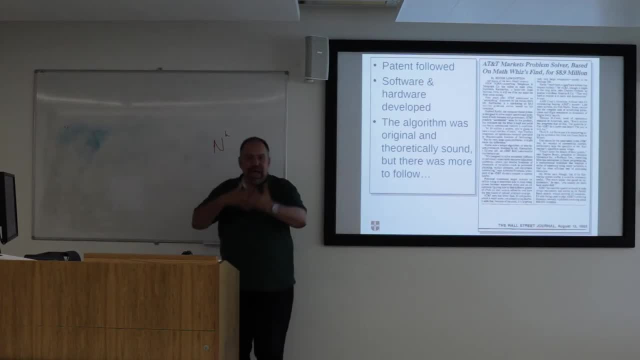 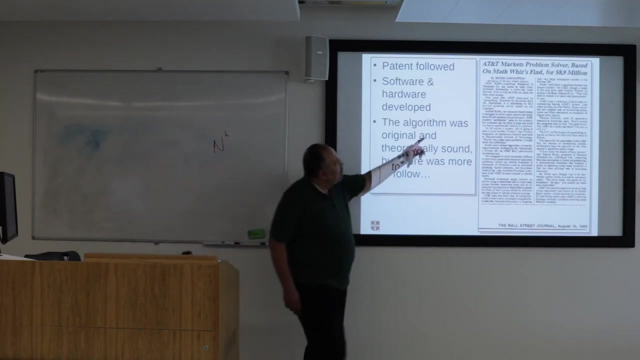 more to follow. So it seemed like there was a little avalanche around the early 80s happening in this area So well, and you can see for how much. they were marketing their solver for 8.9 million dollars at the time, And this is from the Wall Street Journal. 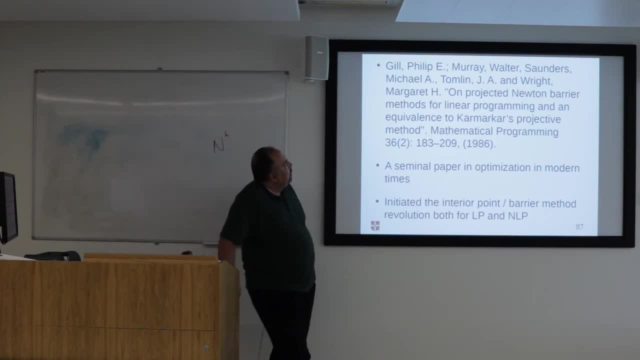 Then came this paper by Gil Murray, Saunders and Tomlin and Margaret Wright where they showed this was a seminal paper- where they showed equivalence, basically of Karmaker's method to a class of problems that was already known from the 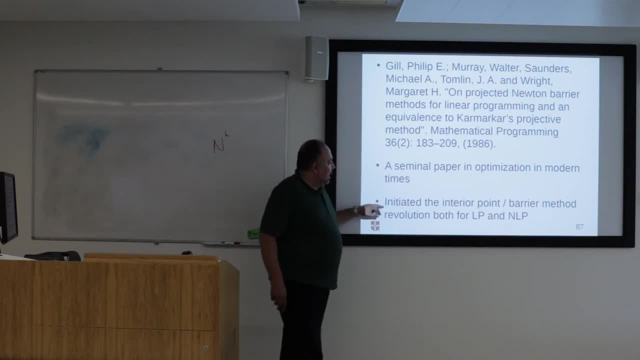 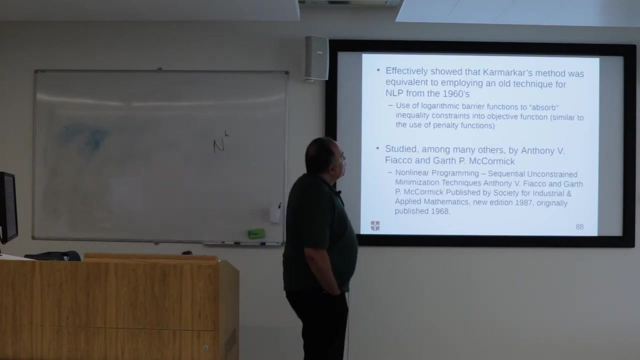 1950s, and we'll see what it was. It initiated the interior point barrier method revolution both for linear programming and non-linear programming in 1986. So effectively they showed that Karmaker's method was equivalent to employing an old 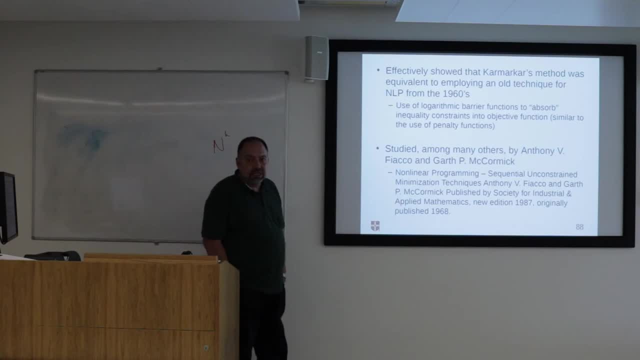 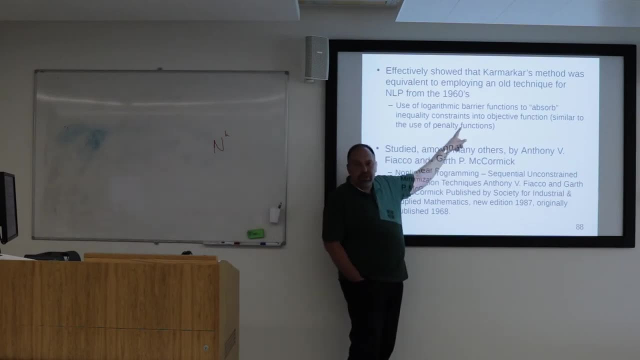 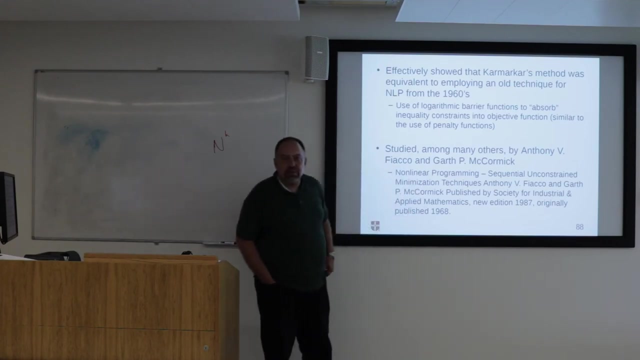 technique from non-linear programming from the 1960s, which is to use logarithms to absorb the inequality constraints into the objective function, penalize them and then solve this problem with a more advanced numerical method, linear algebra. The ideas are published fully in 1968, but the connection was not made and the polynomial 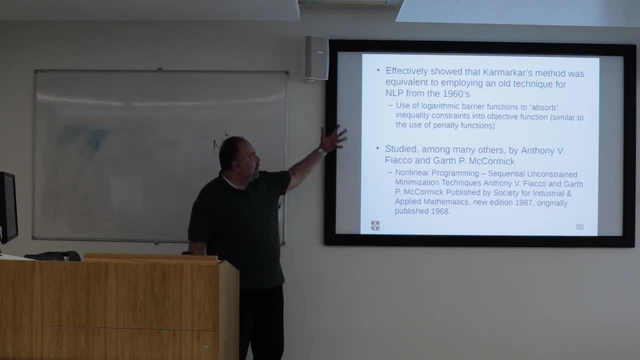 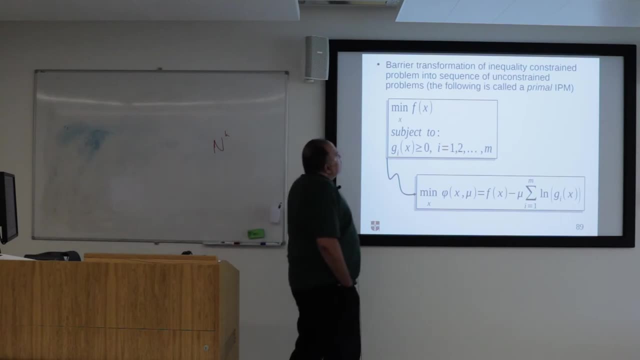 time, complexity was not known until all this was connected together in 1986.. So the barrier transformation of an inequality-constrained problem into a sequence of unconstrained problems follows this logic. Let's say we have an objective function f of x and we have an equality of g i greater. 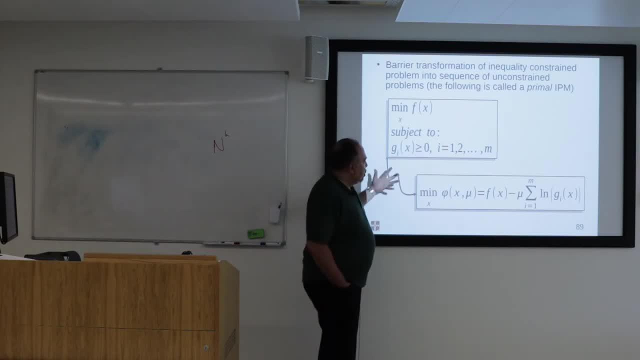 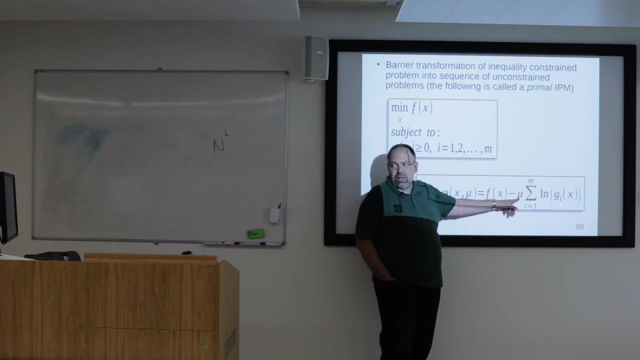 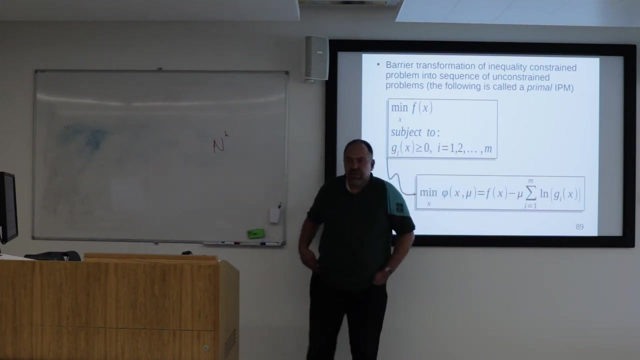 than zero. The way we turn it into an unconstrained problem is by using a barrier parameter mu, a barrier parameter mu and summing up all the logarithms. So we're going to use a barrier parameter mu of the inequality constraints which have to be strictly feasible. 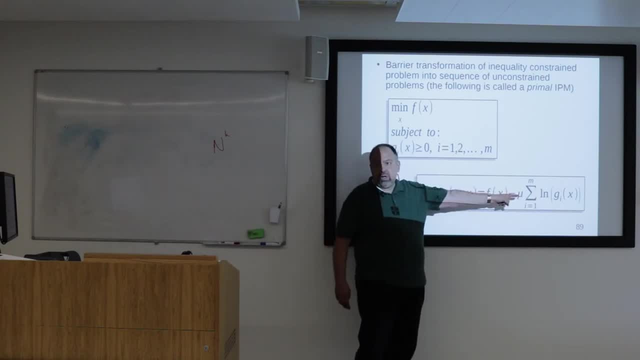 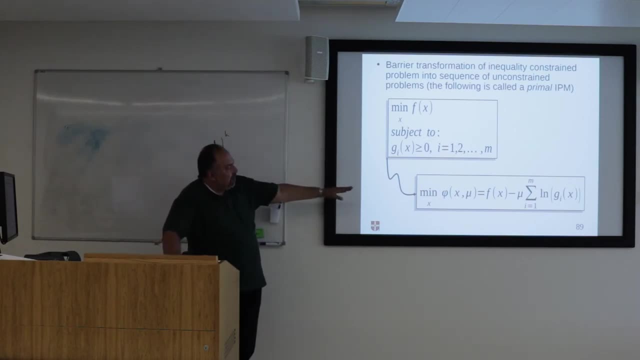 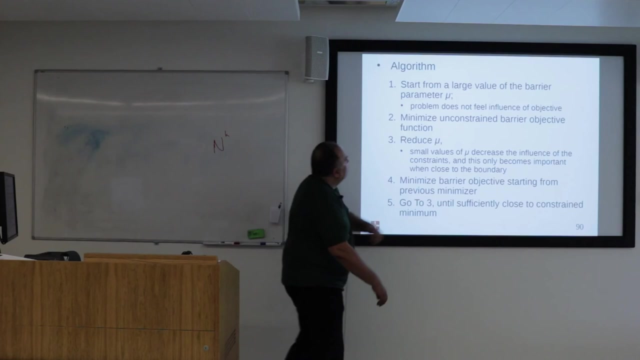 Otherwise you wouldn't be able to plug in here a negative number into the logarithm. So this reformulates the constraint problem into an unconstrained one. So the algorithm starts from a large value of the barrier parameter mu, where the problem does not really feel the influence of the objective. 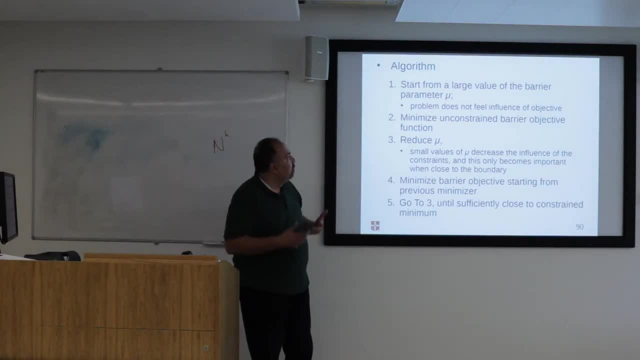 it's a big value of mu penalizes heavily the constraints. Minimize the unconstrained barrier objective function not with standard, unconstrained algorithms, but with suitably tailored routines. Reduce your mu and small values of mu. decrease the influence of the constraint. 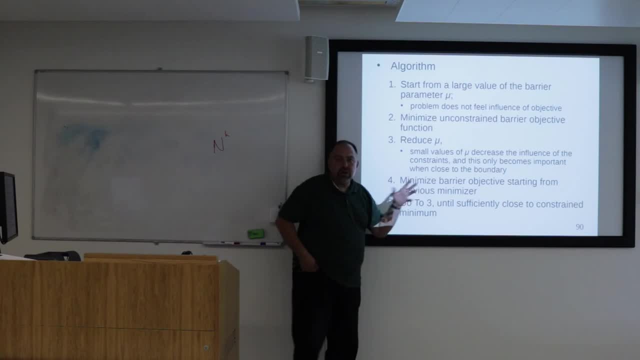 and this only becomes important when close to the boundary. So when you're close to the boundary, the logarithm becomes very, very large, repelling you to go inside And minimize the barrier objective, starting from the previous minimizer, and go to step three. 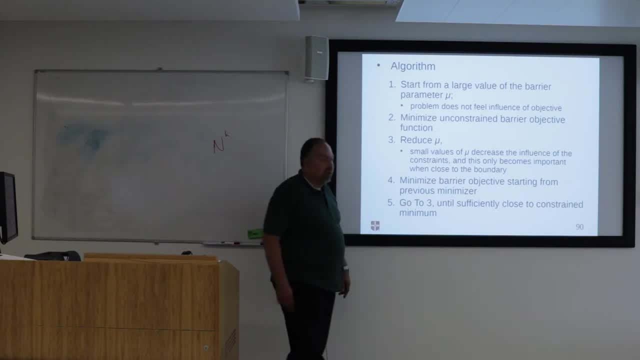 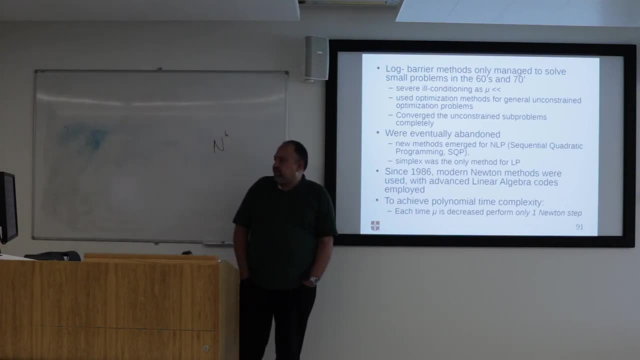 where you reduce your mu until you're sufficiently close to a constrained minimum, And let's see an example later Now. the issues were that log barrier methods only managed to solve small problems in the 60s and 70s and they were abandoned basically from then on. 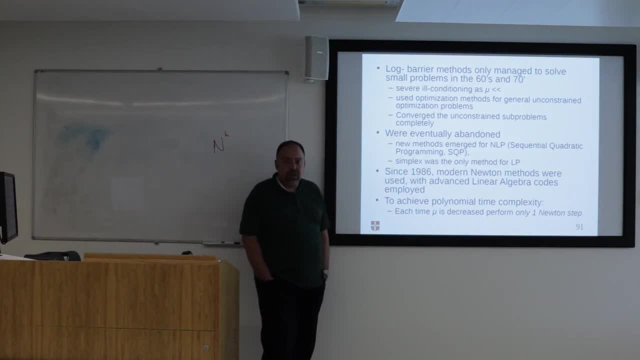 because of the severe ill conditioning as mu becomes very small. They used standard optimization methods for the unconstrained problems, which was the mistake or the problem, and they converged the unconstrained problems completely, which also required extra effort. These were eventually abandoned as new methods emerged for 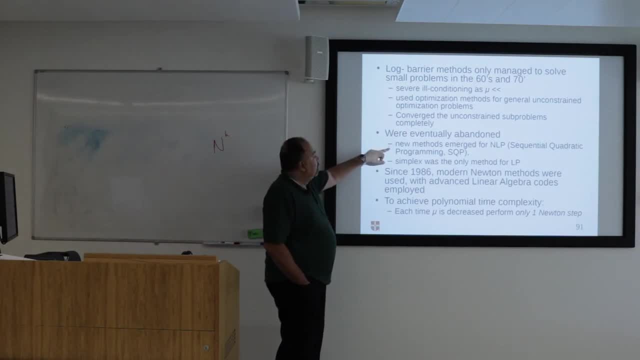 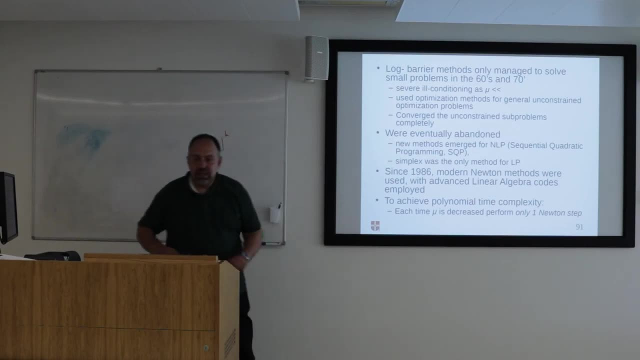 for non-linear programming, sequential quadratic programming, for example, And simplex was the only viable method for linear programming up to that point. Yes, Can I ask a question? Yes, Brilliant. So does the use of the, the barrier, the logarithmic barrier, function in this case? 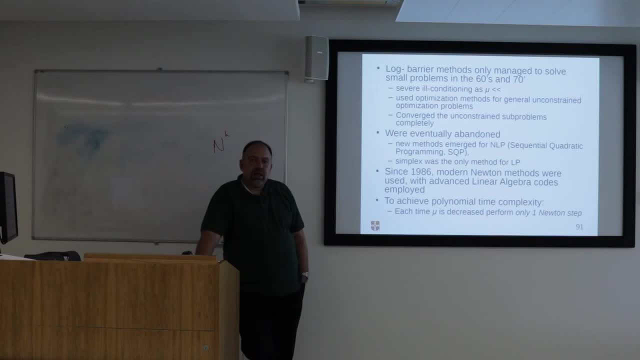 guarantee that you end up with an objective function which is compact over the area that? you're-. No, So your constraints have to be convex and your objective has to be convex. Oh right, Okay, So if you start from a convex programming problem, 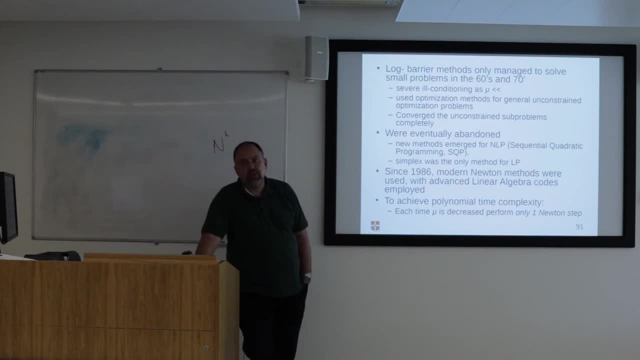 the logarithmic transformation is convex and it will preserve it and you will have only a unique minimum. But if you start from G, the inequality is not being convex or the objective not being convex, then you could have problems. All right,